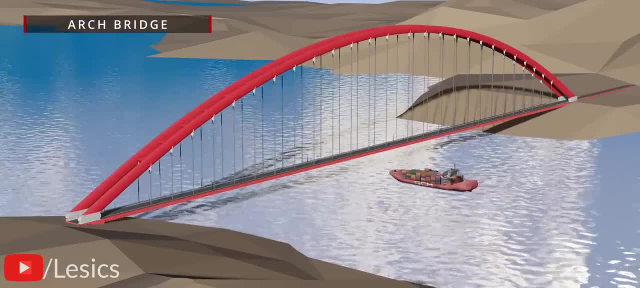 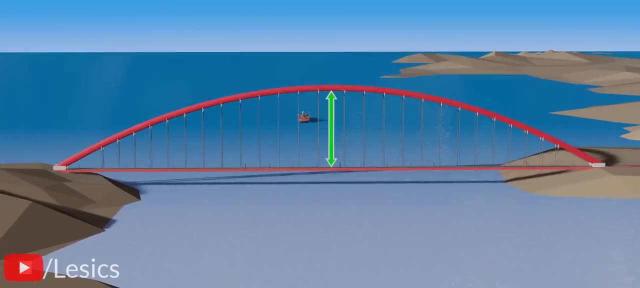 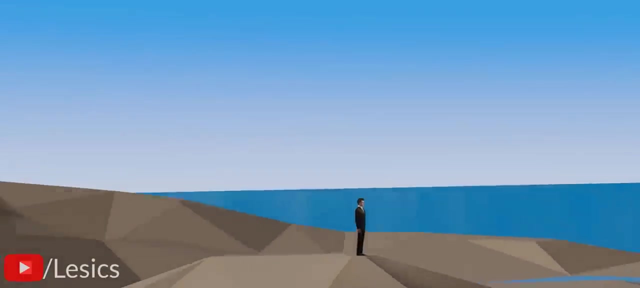 This would definitely provide passageways for ships. However, to maintain the arch shape, the bridge would need to be extremely high. Such a structure would be quite complex to construct. That's why Mr Joseph Strauss opted for a suspension design, a bridge that could overcome all the drawbacks we discussed in a very efficient way. 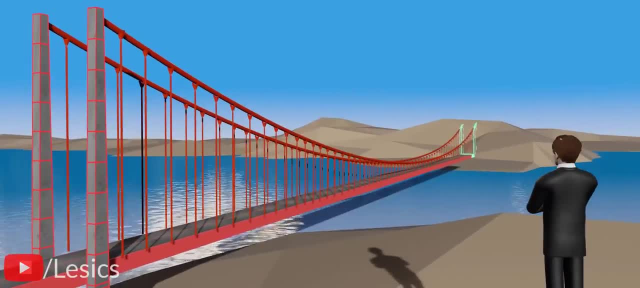 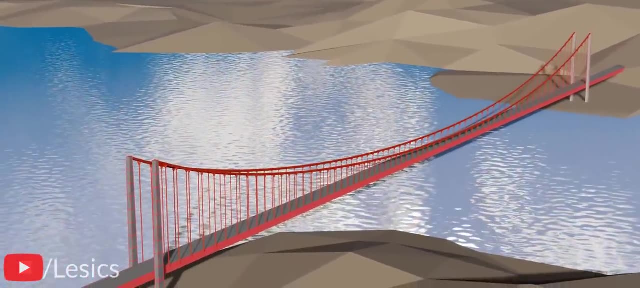 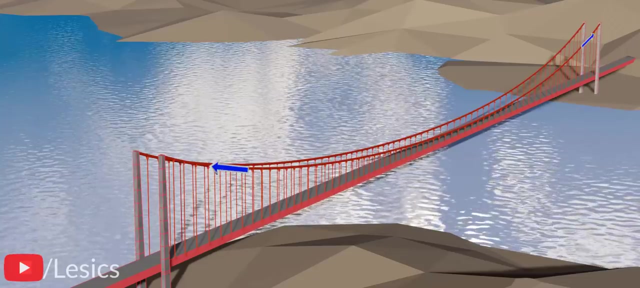 Now let's get into the design details of the suspension bridge. This design has one glaring issue. If you construct the bridge like this, the towers will bend inward. as shown, The main cable is under a huge tensile load. This applies force on the tower. When you resolve this force, you can see that there. 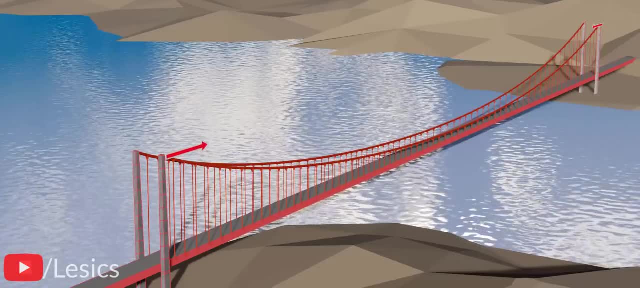 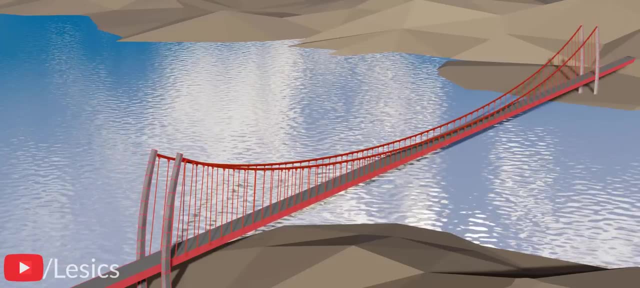 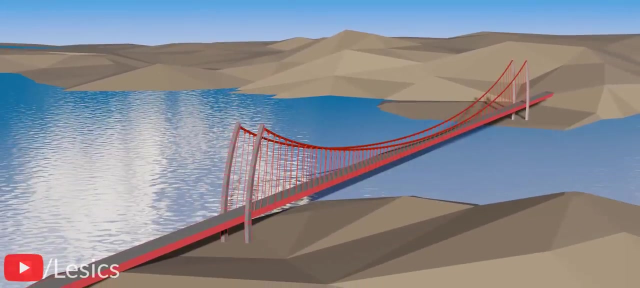 is an imbalanced horizontal force acting inward on the tower, which explains why the towers bend. Can you find a solution for this issue? To cancel this horizontal force, we need the same force acting in the opposite direction. The straightforward solution is to extend the main cable and anchor it down to the ground via an anchorage system. 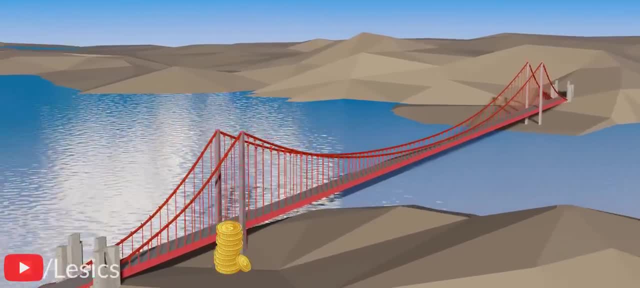 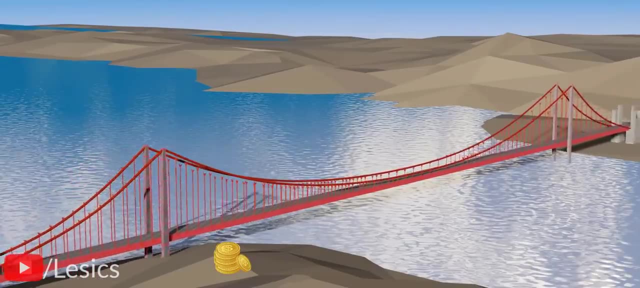 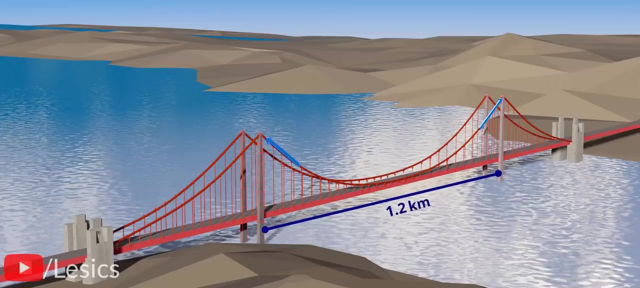 However, we can optimize the financial resources needed to construct this bridge with a simple idea. All we need to do is move the towers closer to one another. Now, the length of the unsupported bridge deck is reduced. Due to this, tension in the cable will be reduced. 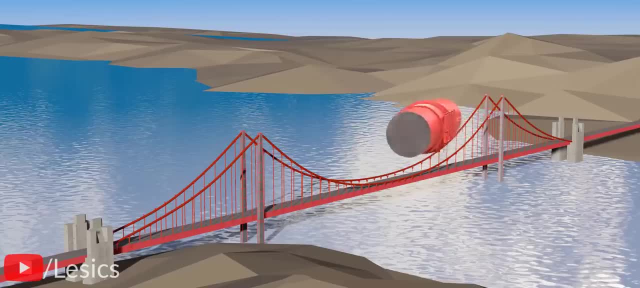 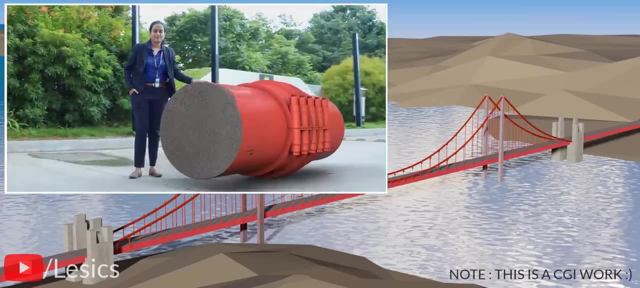 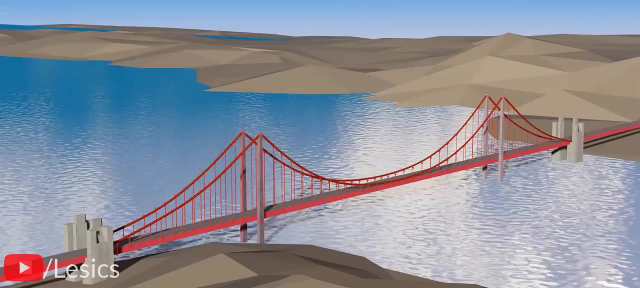 This will obviously lead to a cable with less cross-section area. The width of the main cables are more than half the height of the average human. As a tourist attraction, a piece of this impressive main cable is demonstrated near the Golden Gate Bridge. However, if you construct the bridge with this exact design, it will experience a premature. 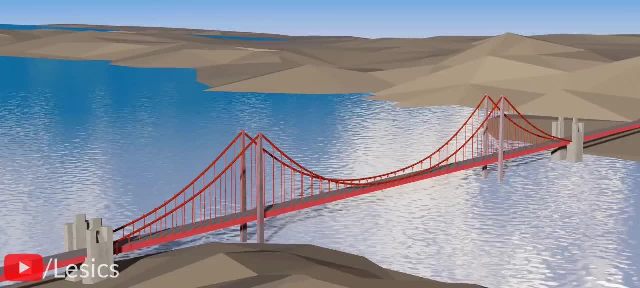 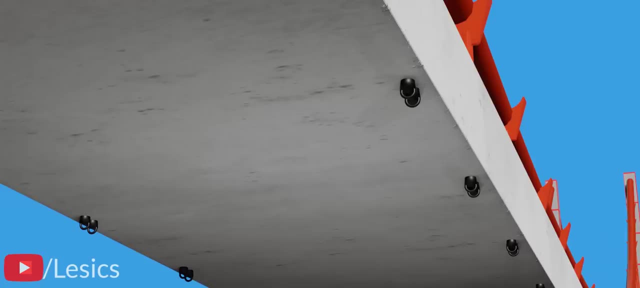 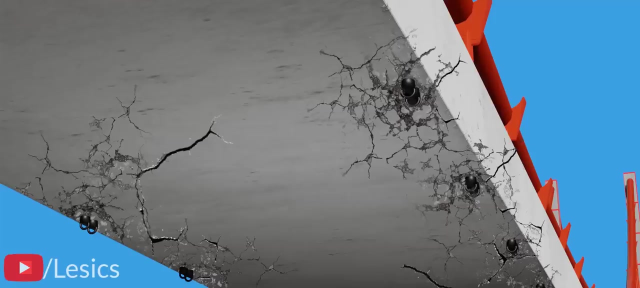 death. Can you guess why this would be the case? Connections are the weakest part in any structural system. The direct connection of the steel suspenders with the concrete deck will lead to the formation of cracks on the deck, since concrete is brittle in nature. 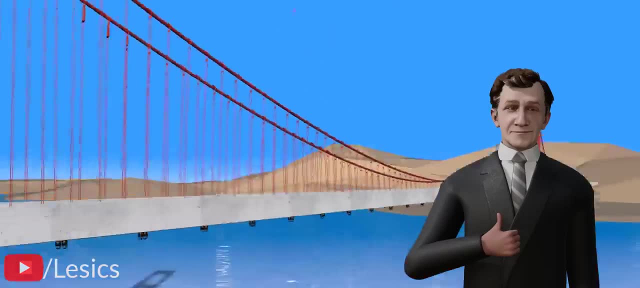 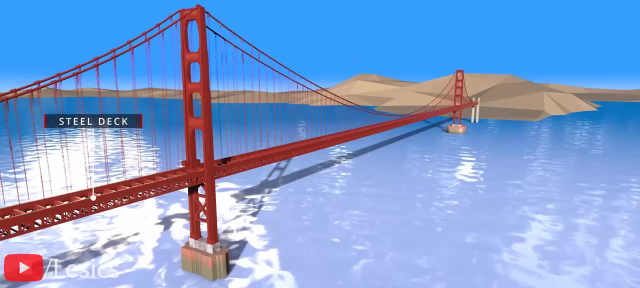 Let's see how Mr Strauss solved this problem. Mr Strauss decided to build a bridge with a single cable. He decided to connect the suspenders to a steel structure. Steel-to-steel connection is always strong. The details of the connection between the suspenders and steel structure are illustrated. 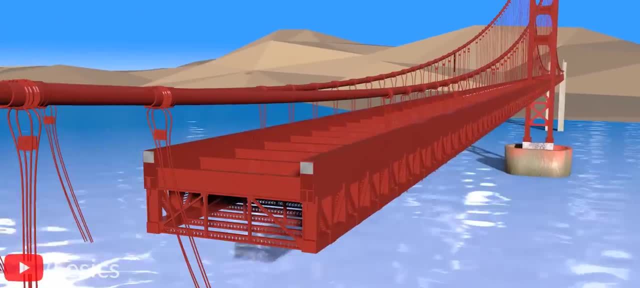 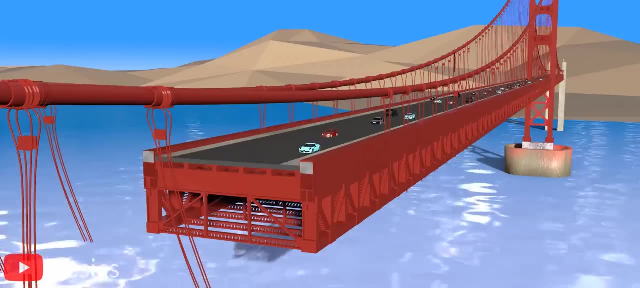 here The road deck is placed on this structure. Mr Strauss kept the width of the road to 27 meters to account for current and future traffic demands. Assembling the structure like this was far from an easy task, due to foggy and windy conditions. 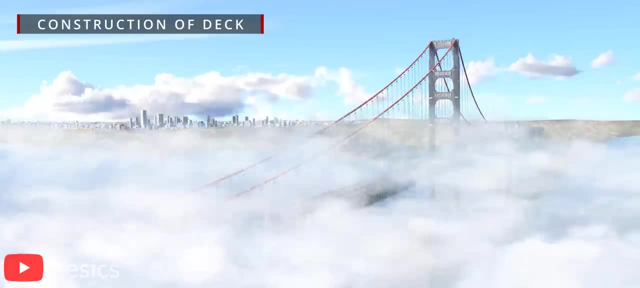 The structure was designed to be able to withstand heavy traffic. The structure was designed to be able to withstand heavy traffic. The structure was designed to withstand heavy traffic. Therefore, the breakpoints and the �yes were determined. Finally, the structure was redesigned for new conditions at the site. 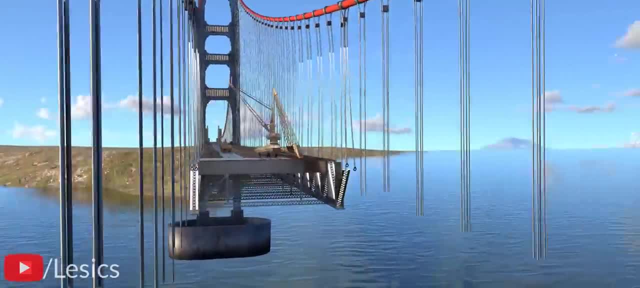 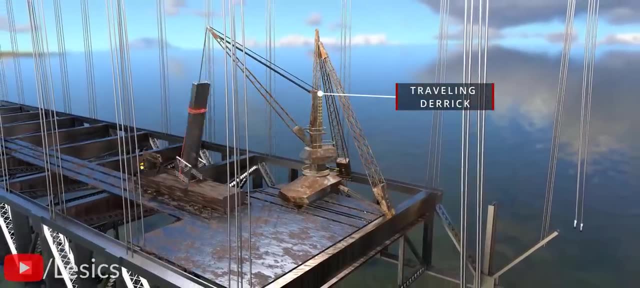 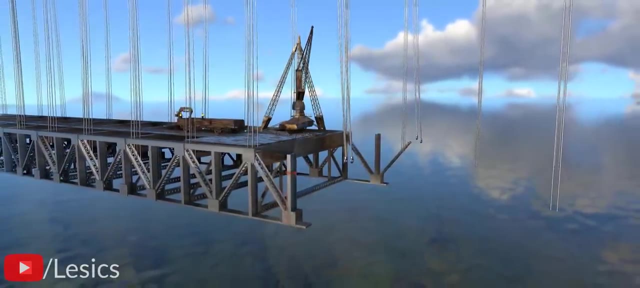 To facilitate the process, workers prefabricated each member of the truss and brought them to the site via ships. Simply, the two men who assembled by usingune daggers would theenz commerce. To ensure the safety of the laborers, a net was installed underneath the bridge deck. 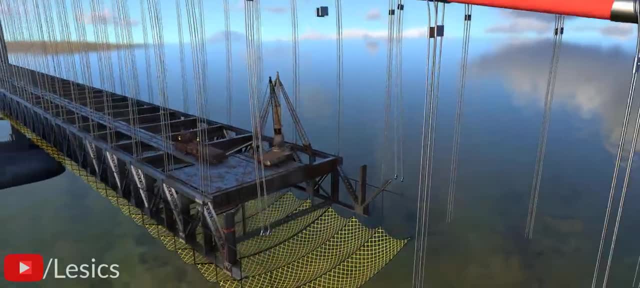 The construction of the bridge was made by the埡ringed leasers. The approach is to bring a Renaissance construction with cables and a progressive steering and some of the vertical joints between two sectoric bridge level. Next I'll explain some of the consequences of drownings outside of the structure. 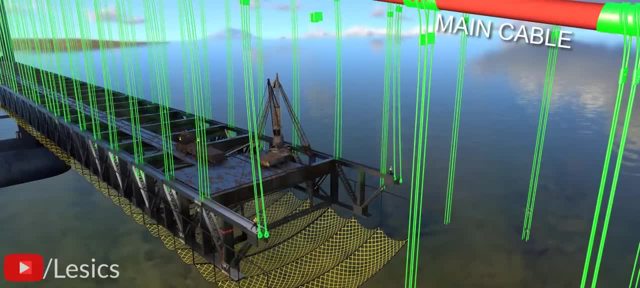 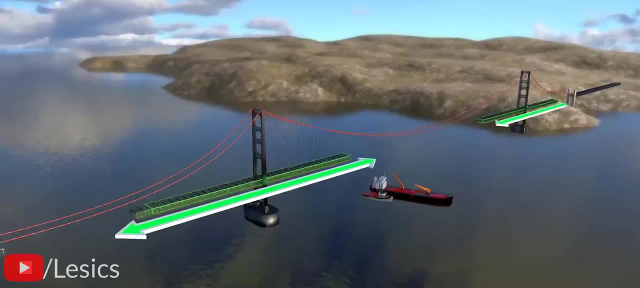 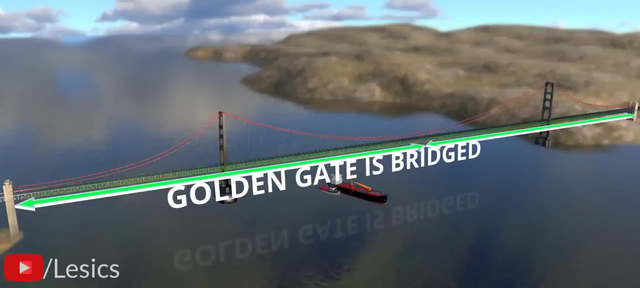 Potholes were placed on a weak concrete structure cables. Moreover, to maintain equal loading on the cable, workers had to assemble the system simultaneously and equally in two directions for each tower. Thus the Golden Gate was bridged. 250 pairs of vertical cable were used and they hung the whole bridge deck to the main cable. 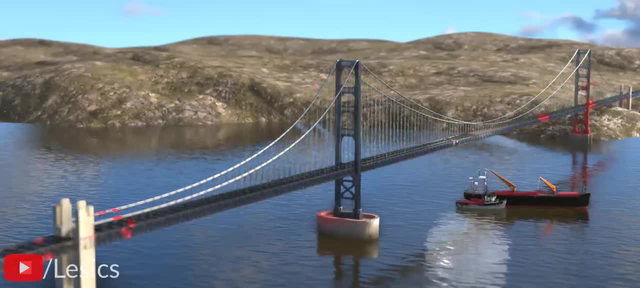 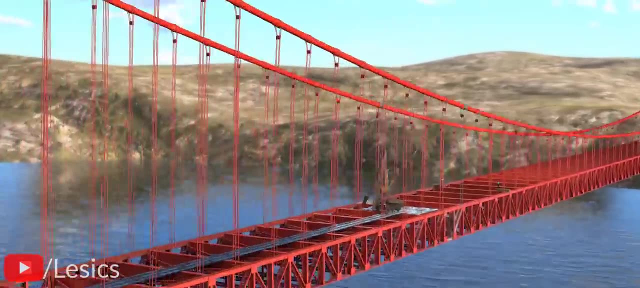 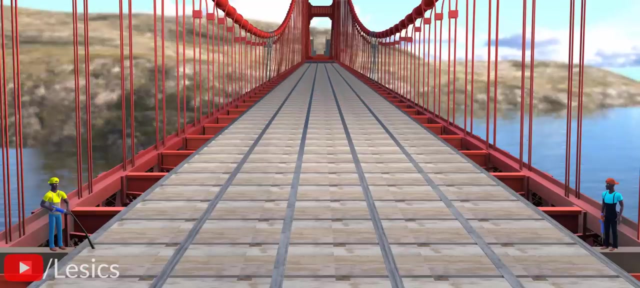 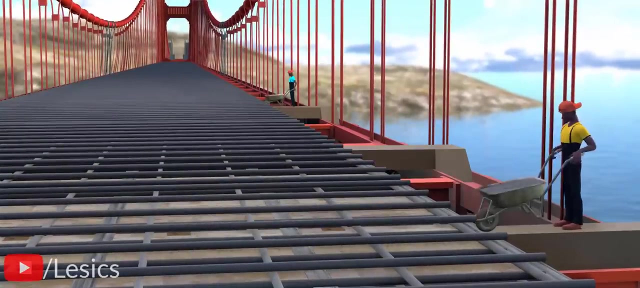 After the construction of the steel structures, the workers painted the bridge a special international orange color. Next, let's examine some details of concrete road construction. on top of this solid structure, Workers first laid down wooden formwork. They attached steel bars, welded them to the steel sections below them and later poured and compacted the concrete. 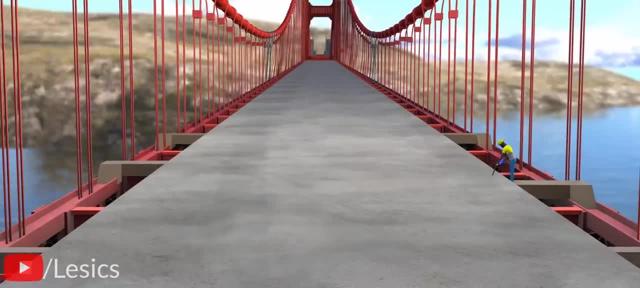 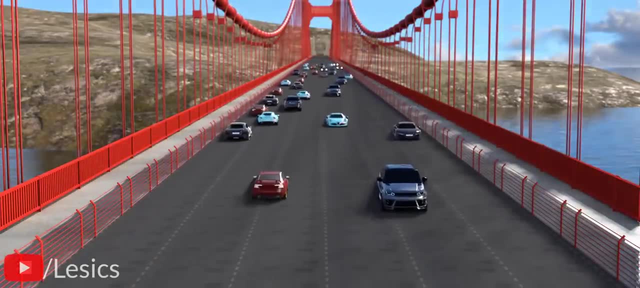 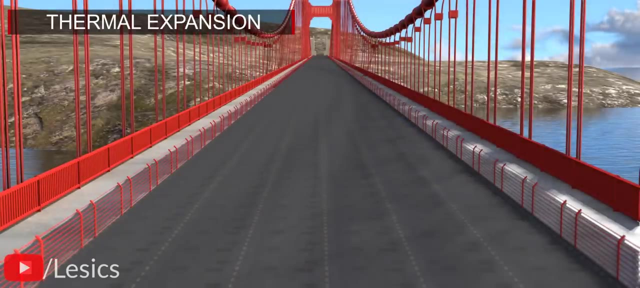 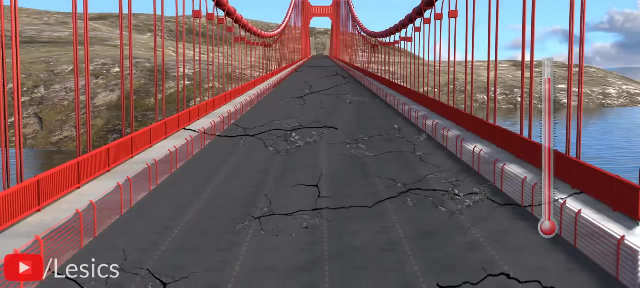 using a needle vibrator. Our bridge looks perfect now, but is it ready to support vehicles? Not yet. We must first tackle another major engineering challenge: Thermal expansion. The concrete and associated steel structure will expand or contract based on environmental temperature variations If we had constructed this bridge as a single piece during a hot, sunny day. 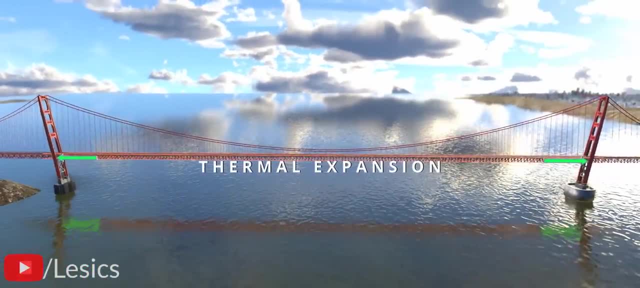 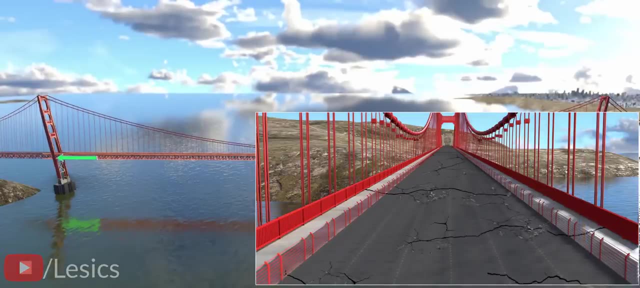 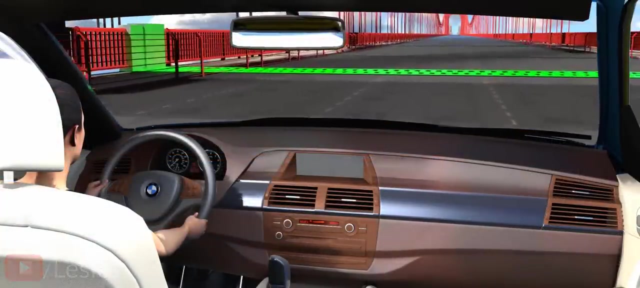 the bridge would expand and cause tremendous stress on the tower as well as on the road. Eventually, the bridge would experience downpour. If you have ever visited the Golden Gate Bridge, you may have noticed peculiar connections on the road. These connections, called finger expansion joints, were Mr Strauss's solution to solve. 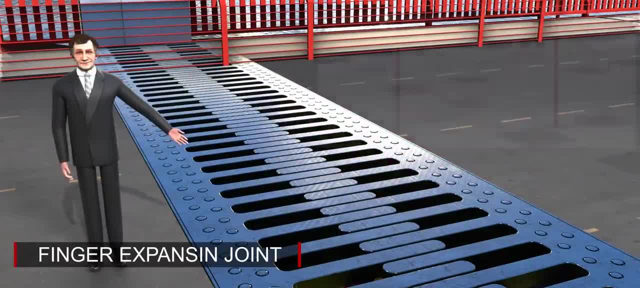 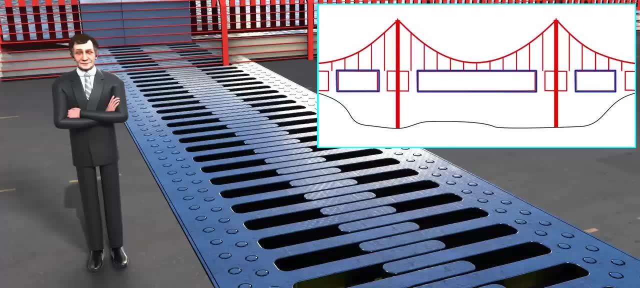 the thermal expansion problem. Mr Strauss divided the deck into seven separate pieces. You can see this bridge has three cradles. The finger expansion joints are installed between the gaps. The thermal expansion joints are installed between the gaps During an extreme temperature. 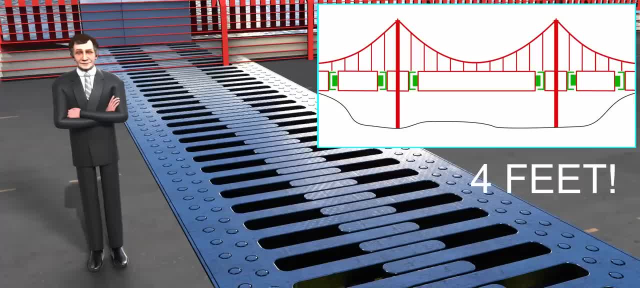 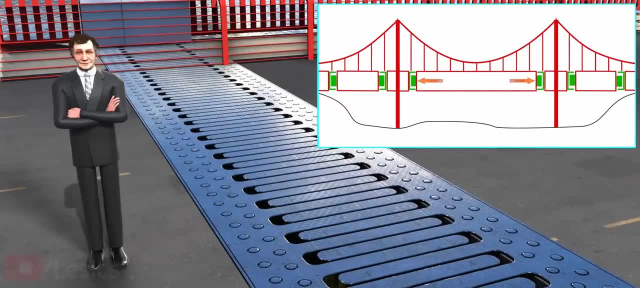 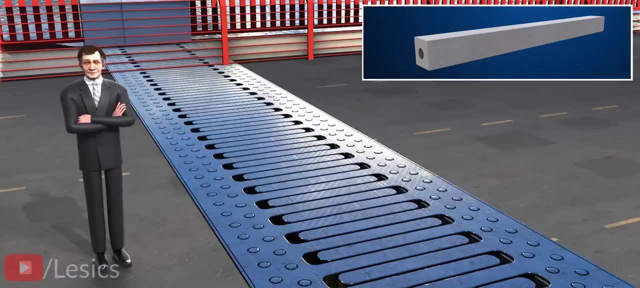 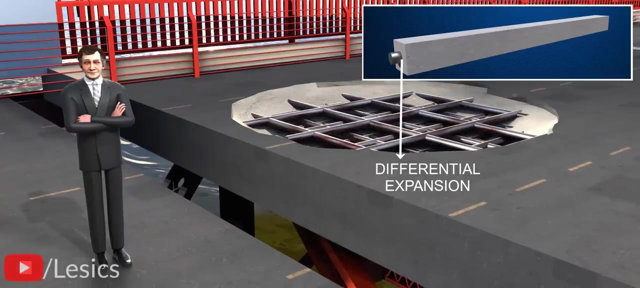 the length of the deck is increased and these joints move by almost four feet. I think all technology should be strict about interospel warfare, such as the thermal expansion control. What an elegant solution for a serious issue. However, there is still a small problem to solve. 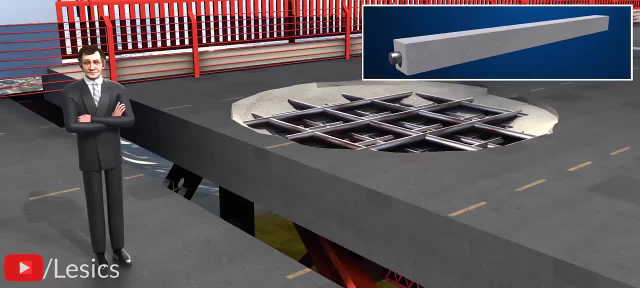 The thermal expansion of the steel is slightly higher than that of the concrete. This differential 1999 Analogimo 9- cauemos expansion can cause trouble for the concrete deck, which is composed of a mixture of concrete and steel bars- boy bars- but this expansion issue is negligible when the length is small. 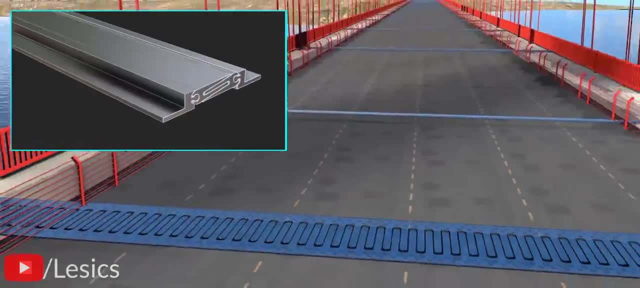 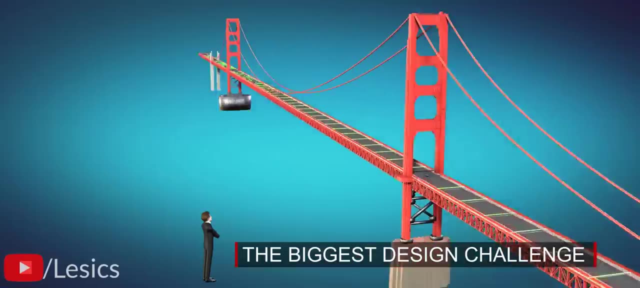 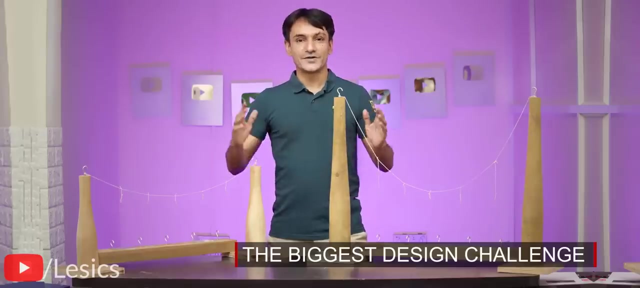 This is why the Golden Gate contains tiny expansion joints every 50 feet. Another great design challenge Mr Strauss dealt with was the height of the tower. Let's do an experiment to gain a better understanding. I have two bridge designs with me. a tall tower design. it is having a high sag and 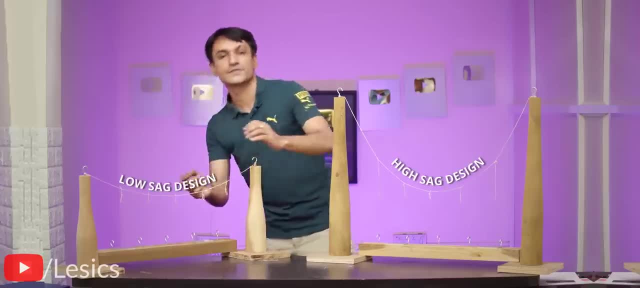 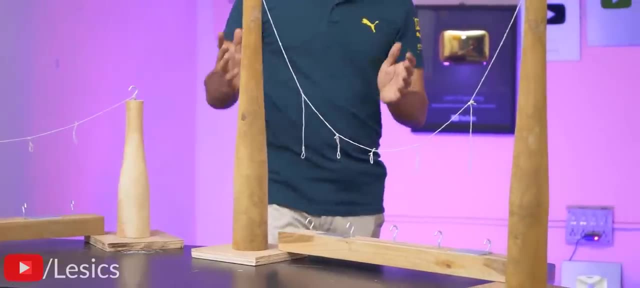 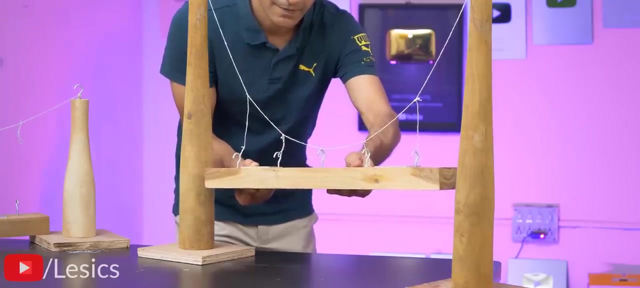 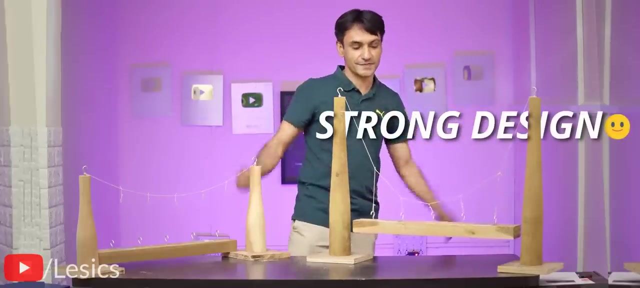 the next one, a short tower design, obviously a small sag. The question is that which design gives more strength to a suspension kind of bridge? Let's test the first design using a rod deck- that too, a really heavy rod deck. When I attach the rod deck, this design is standing strong. this design is safe. 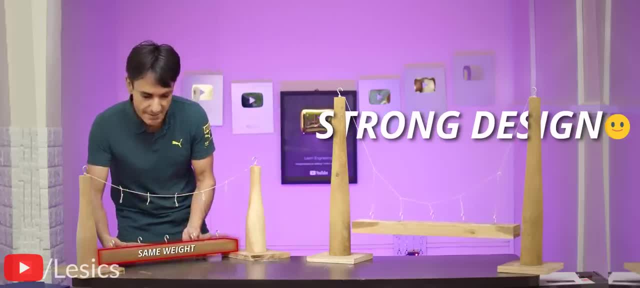 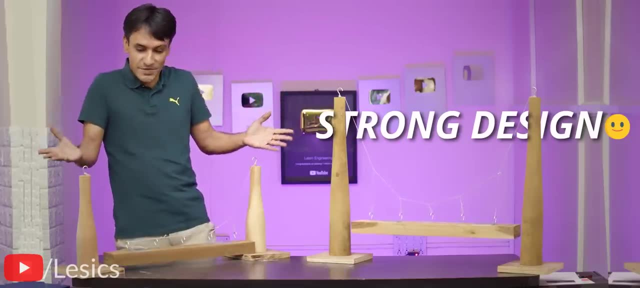 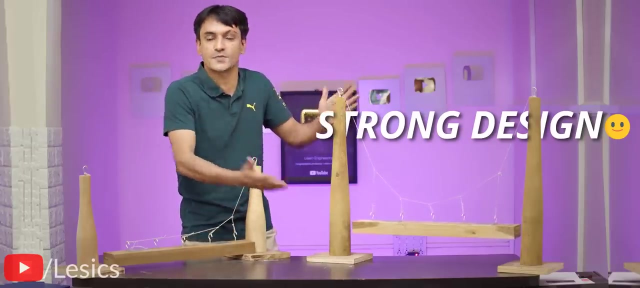 Now let's attach the same weight to the next design, to the short tower design. This bridge went for a sudden failure. I couldn't even react to that. So in short, we proved experimentally: the tall tower design is the best for a suspension. 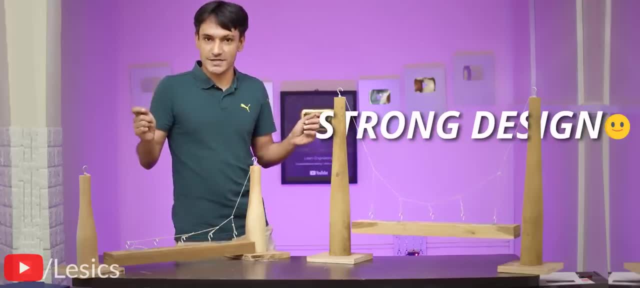 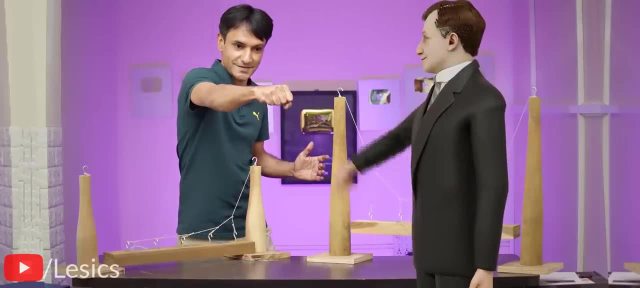 kind of bridge, it's more strong. The question is why? To get answer for this, let's invite the chief engineer of this whole project, Mr Joseph Strauss, to the video. The major difference between these two designs is the angle of the cable. 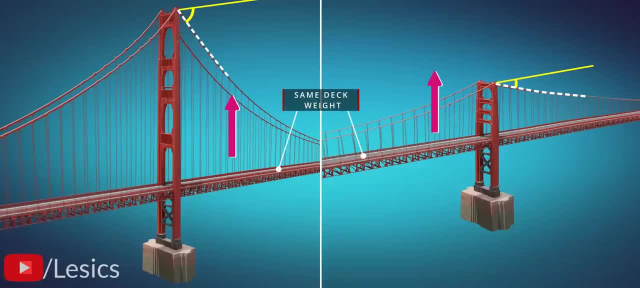 In both the load to be carried is the same. The vertical component of the cable, tension, balances this weight. Since the small tower design has a low angle, to balance the weight, the cable has to induce more tension. This is why the short tower fails during the experiment. 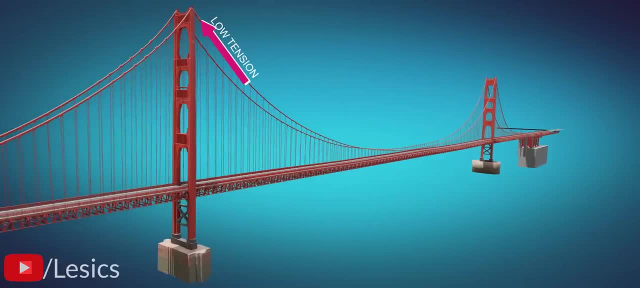 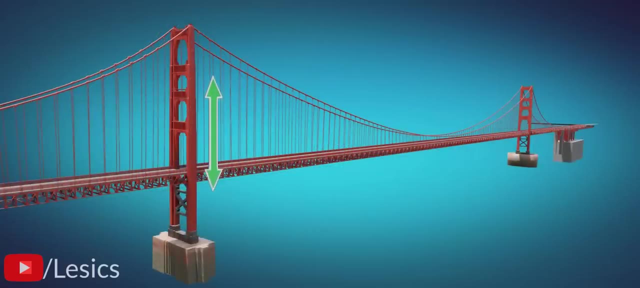 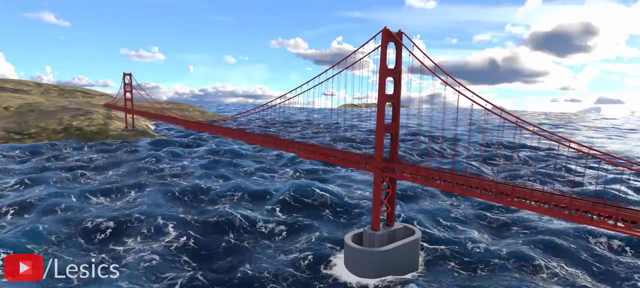 The tall tower will obviously reduce the tension in the cable, but it will cost much more to construct it. That's precisely why Mr Strauss calculated the optimal tower height of 746 feet, A happy average between these two scenarios. Now let's get into the most exciting part of this video. 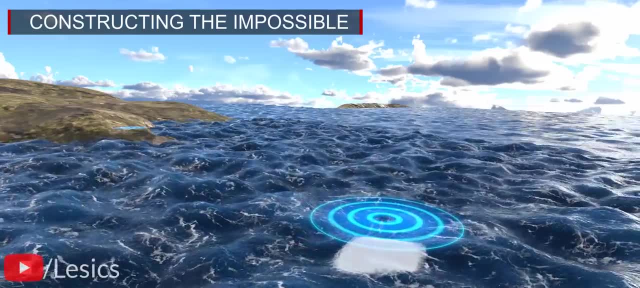 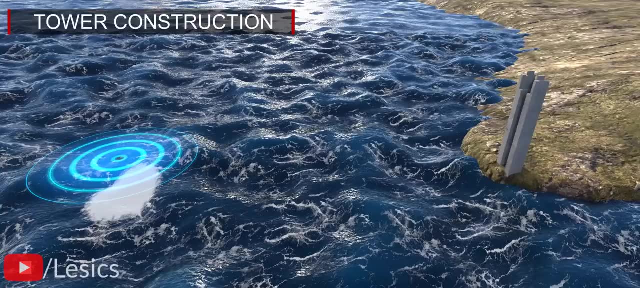 Construction of the Golden Gate Bridge in a hostile environment. First we start with the tower construction. Did you know the construction of the Southside Tower was tougher than the North Tower? This is because the South Tower construction had to overcome the violent Pacific Ocean. 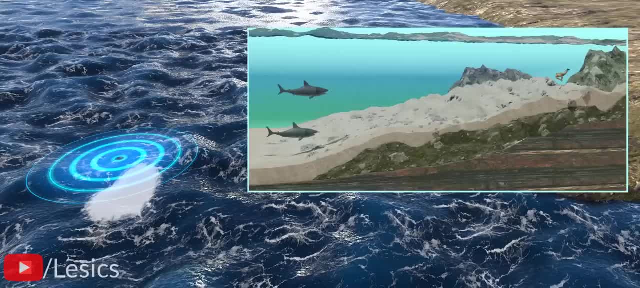 A tower foundation must be constructed on strong bedrock called a rock. The construction of the South Tower construction had to overcome the violent Pacific Ocean. A tower foundation must be constructed on strong bedrock called a rock. This is because the South Tower construction had to overcome the violent Pacific Ocean. 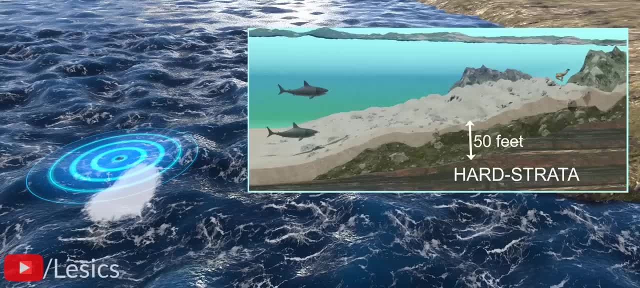 The construction of the South Tower. construction had to overcome the violent Pacific Ocean. For the Southside, the Hard Strata was 50 feet below the seabed level and had a steep floor. For the Southside, the Hard Strata was 50 feet below the seabed level and had a steep floor. 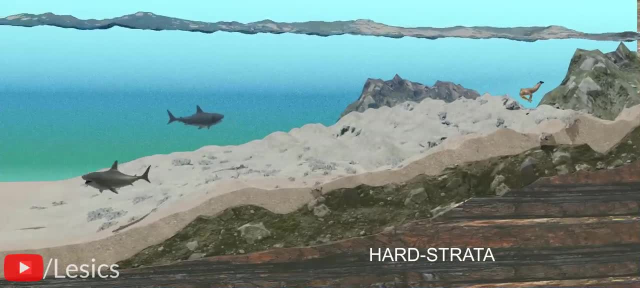 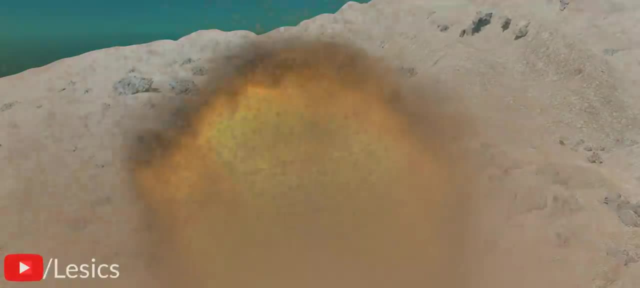 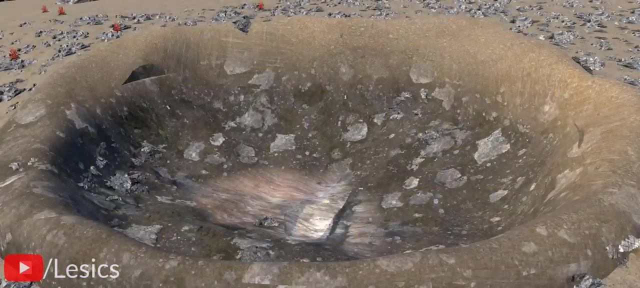 We need to dig this deep and build a RCC foundation for the South Tower. To do so first, professional divers were hired to blast bombs underwater. The divers cleared the debris of the explosion and made a better surface. Now it's time to construct a steel and wooden framework on this surface. 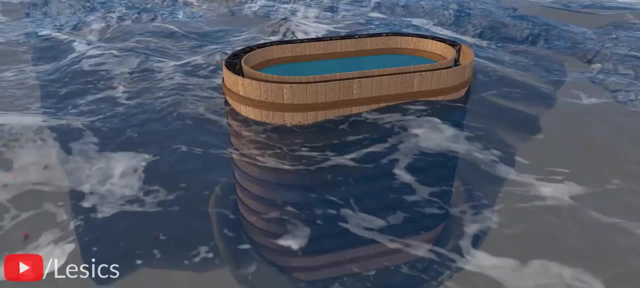 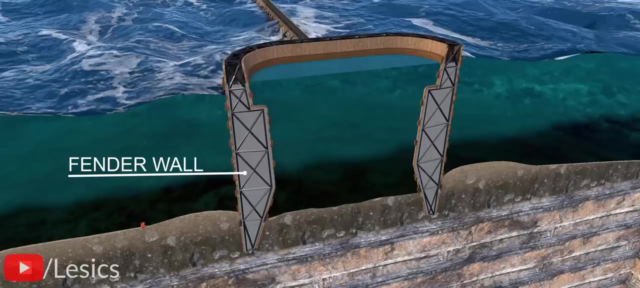 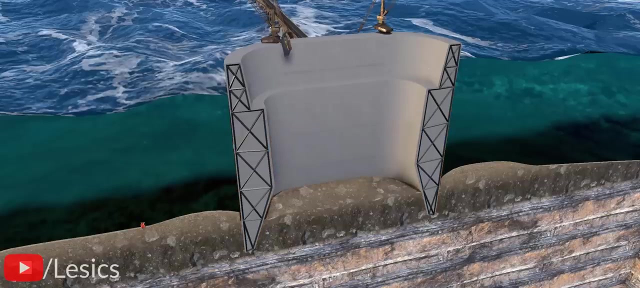 The divers obviously did an amazing job here. Now let's see the cross section of the structure they built. Then the concrete was poured to create something called fender walls. Afterwards all the inside water was pumped out. Now that the fender wall is ready, can the workers go inside? 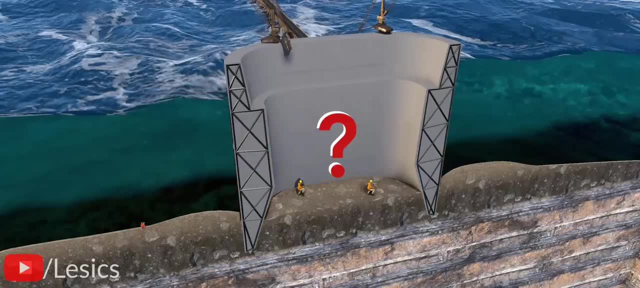 and start digging for the hard strata. Here is the issue: The ocean currents are so nasty that the fender wall will have to bear a huge inward force and can collapse. This kind of construction is highly unsafe. Mr Strauss had a clever idea. Initially they placed the blasting tubes. 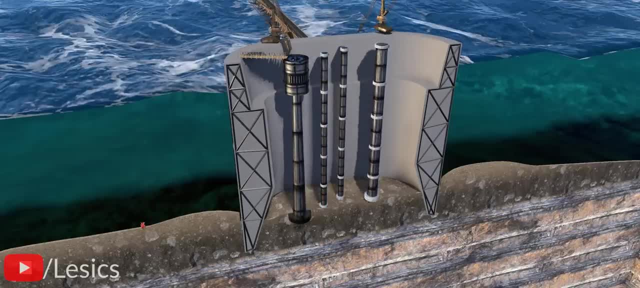 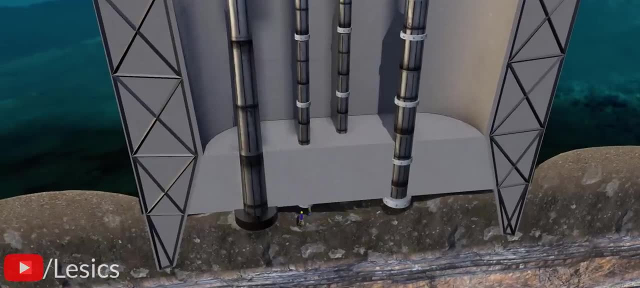 the workers shaft and the material shaft inside the fender walls. The trick was to construct a thick, reinforced concrete slab so that workers can work beneath it. The way workers reached the water was by putting the construction of a thick, reinforced concrete slab, and the workers can. 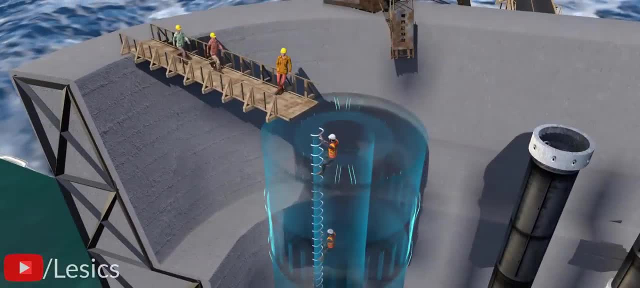 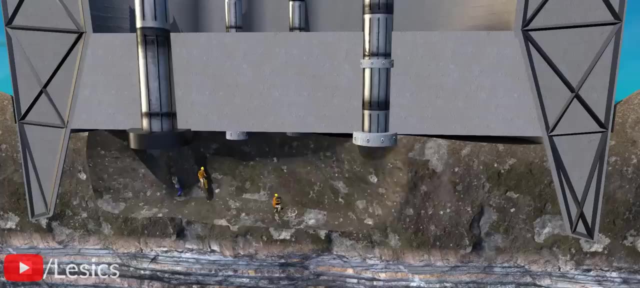 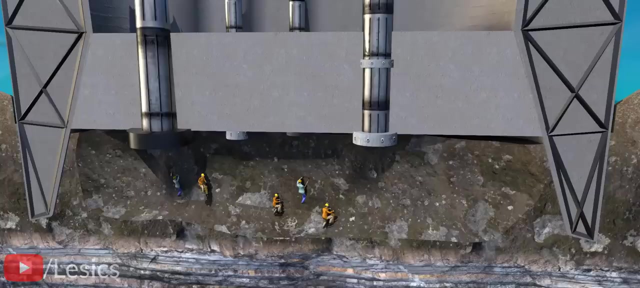 workers' chamber was quite interesting. It was via the workers' shaft. They continuously drilled the boulders and dug underneath the RCC slab. This RCC slab supported the fender walls and protected the workers underneath against deadly currents. During this process, the entire fender 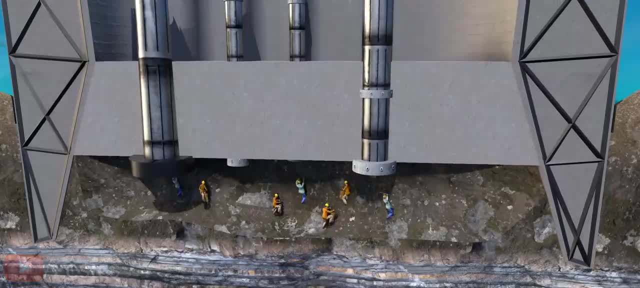 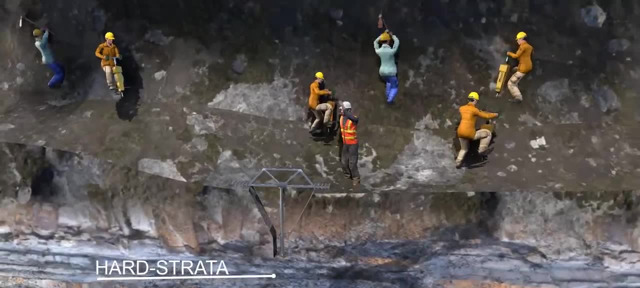 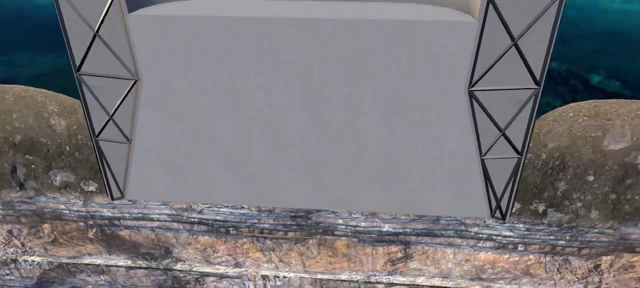 wall structure was allowed to sink slowly. You can see its knife-like shape. Eventually they reached the rocky hard strata. After leveling the hard strata, they made a steel structure there and built an RCC foundation- The construction of the complete foundation. 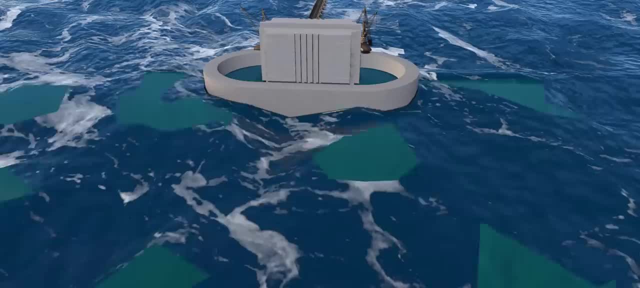 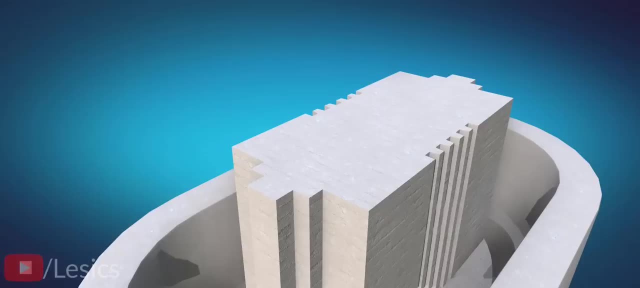 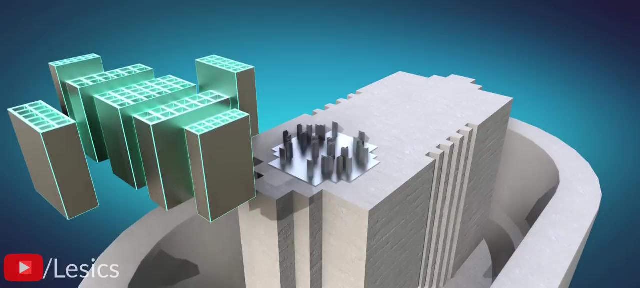 is quite easy. now You can see how the fender walls protect the main foundation from the deadly waves. Now it's time to see the construction of the gigantic towers. Once the foundation was ready, they assembled the steel base plate on it. Now comes the magic. 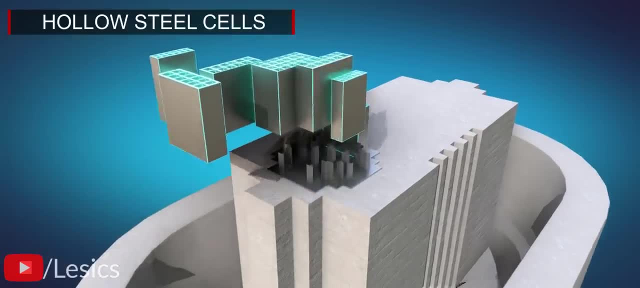 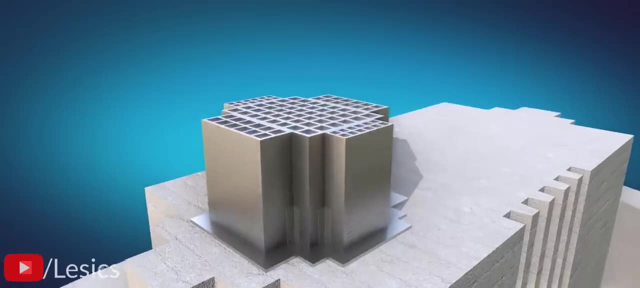 They assembled and riveted these cells as if they were constructing a tower using Legos. You can see how cleverly they had to plan the shapes and sizes of these cells so that the tower would finally achieve the shape which it was intended to achieve. 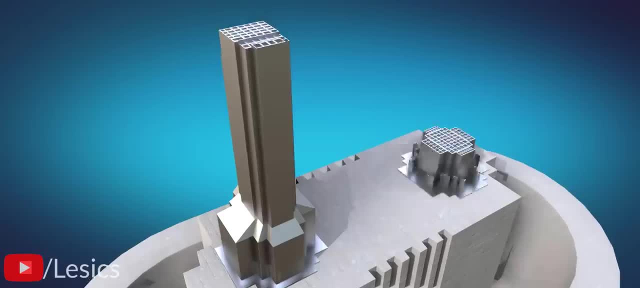 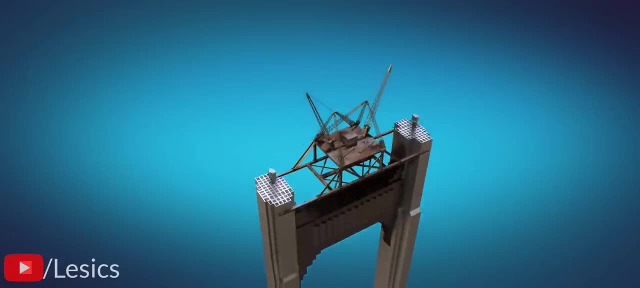 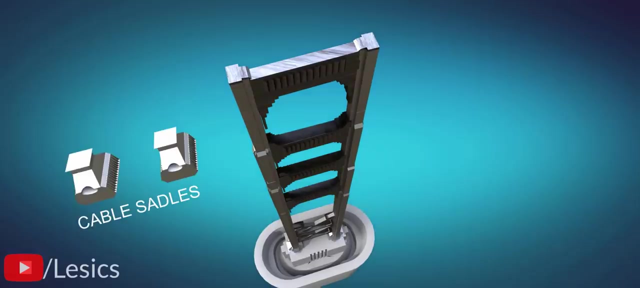 Mr Strauss designed this unique cellular structure to be economical as well as strong. The tower construction was then complete. Next, it was time to level the tower. The first thing this people did was lay down the main cables. For this, they first installed cable saddles atop the towers. 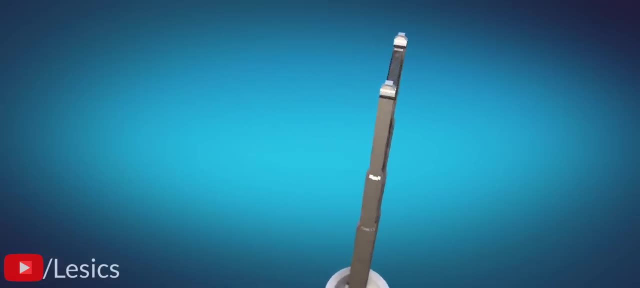 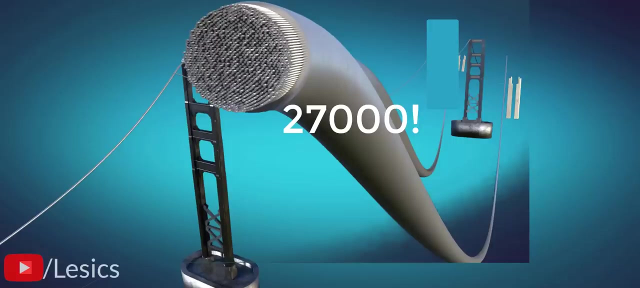 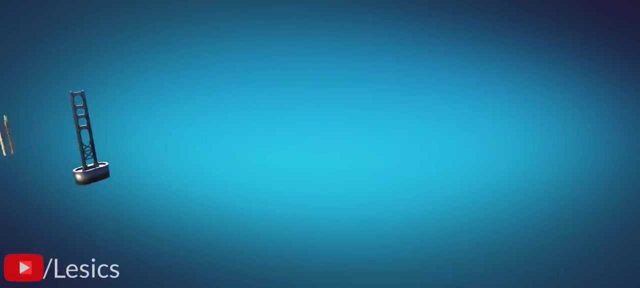 You may think that the main cable is a single solid cable. The main cable is in fact made up of twenty-seven thousand smaller wires and a total length of 129 thousand kilometers length of steel wire was consumed for fabrication of it. To start laying these cables, workers first constructed a catwalk bridge for themselves. 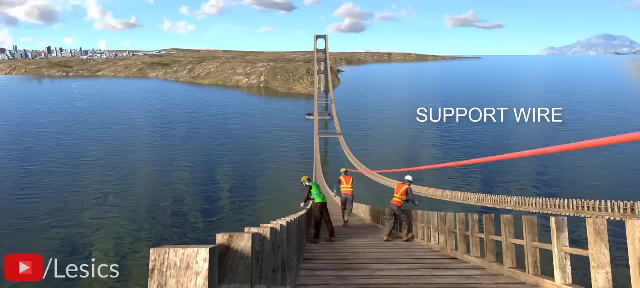 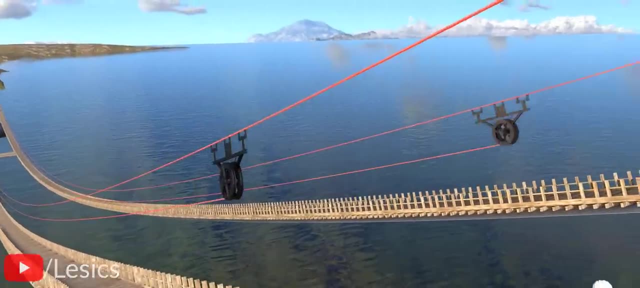 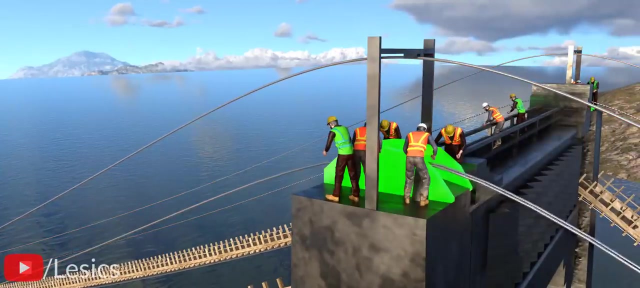 At first, workers laid a support wire. The main cables made their journey via these spinning wheels. Furthermore, these small wires were passed over the tower through the cable saddle, one by one, and were then clamped by laborers. Then the workers pressed the wires tightly using a hydraulic press. 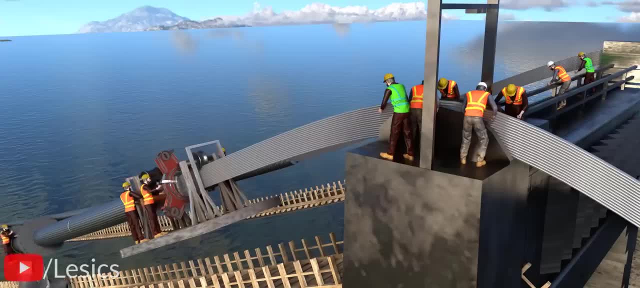 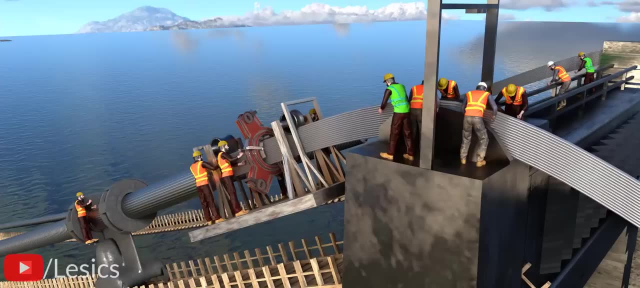 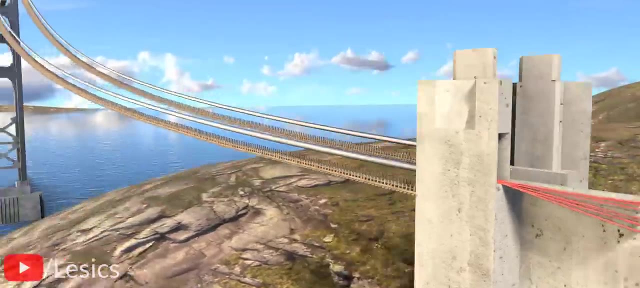 They simultaneously wound the wires together using galvanized steel wire, which is why the main cable looks like a single large pipe. These cables are anchored to the bedrock with strand-shoe steel plates. After laying the main cables, the suspension cables were attached to it. 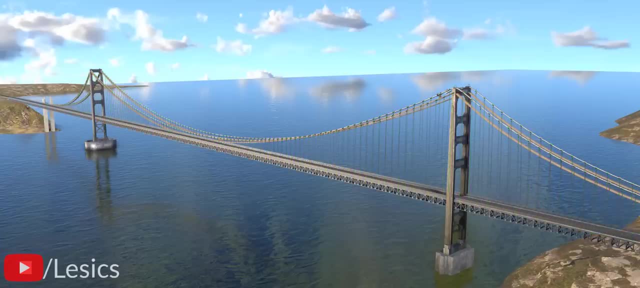 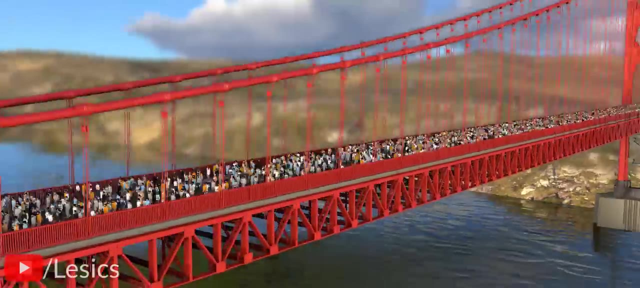 All that was left to do was construct the deck structure and lay down concrete for the road. You already know how they did that. A strange incident happened on the Golden Gate Bridge on its 50th anniversary, when more than 300,000 people gathered on the bridge all at once. 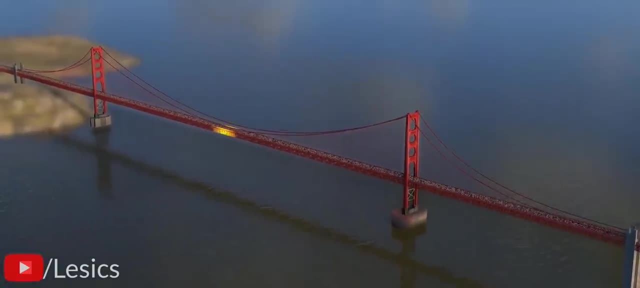 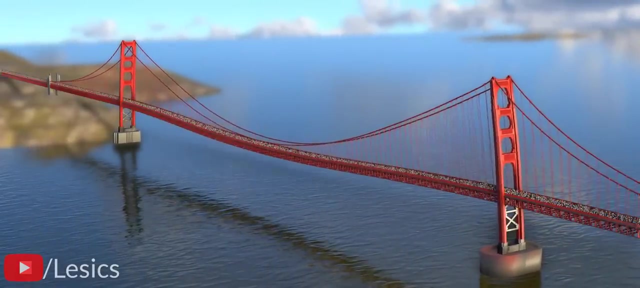 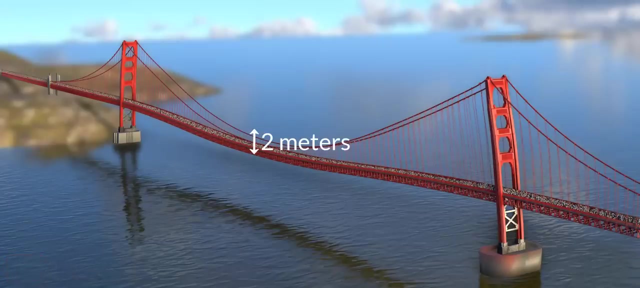 You can probably predict what will happen if a suspension bridge is overloaded. Overloading a suspension bridge can cause it to sag. This can even cause the main towers to bend inward. This is exactly what happened on that day. The road deck sagged by almost 2 meters.